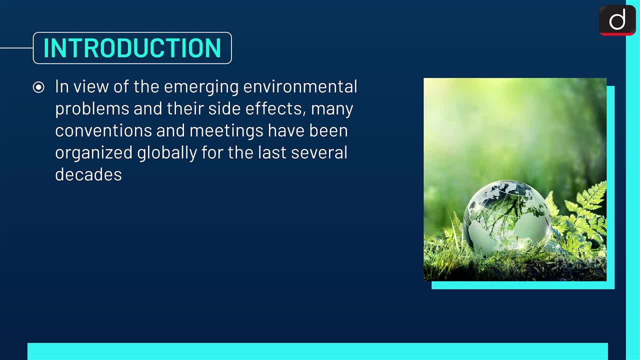 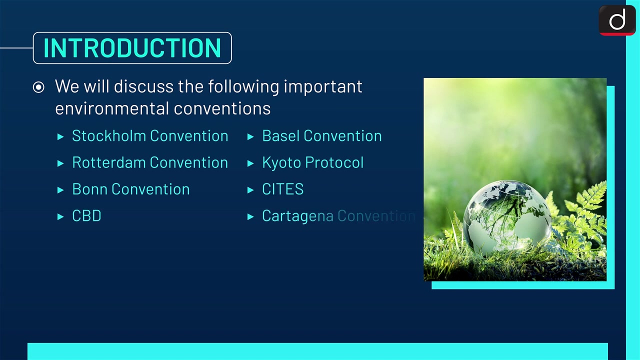 and their side effects. many conventions and meetings have been organized globally for the last several decades. We will discuss the following important environmental conventions: Stockholm Convention, Basel Convention, Rotterdam Convention, Kyoto Protocol, Bonn Convention, CITES, CBD, Cartagena Convention, Minmata Convention and Cartagena Protocol. 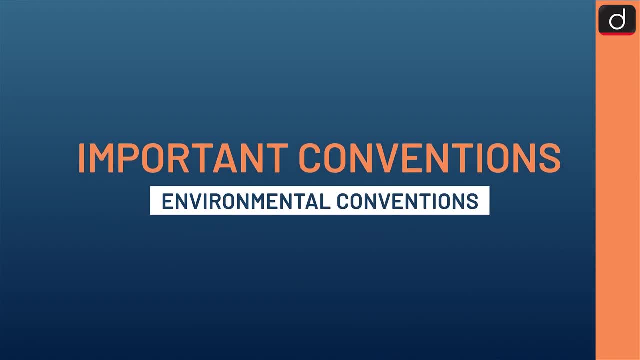 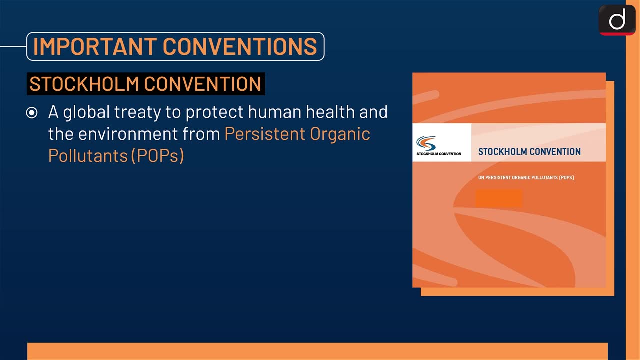 Now moving on to these important conventions, and we will discuss all of these one by one. First is Stockholm Convention. It is a treaty to protect human health and the environment from persistent organic pollutants, or POPs. It was signed on 22 May 2001 and over 152 countries ratified the convention. 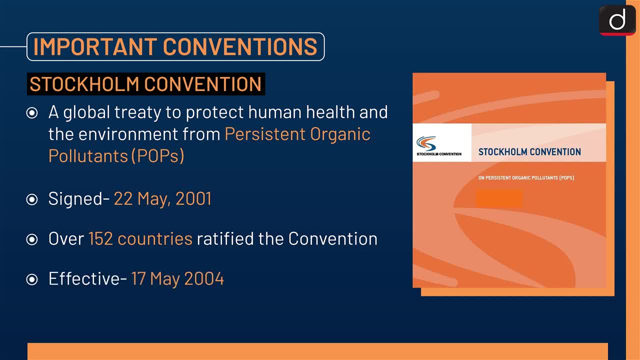 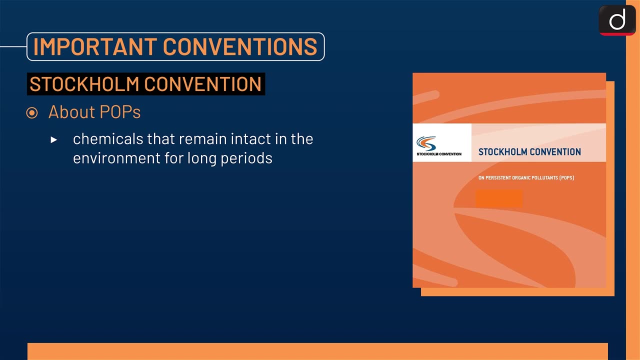 It was effective from 17 May 2004 and was ratified by India on 13 January 2006.. Now let's understand about POPs. Pops are areas that remain intact in the environment for long periods and they are widely distributed geographically. These can reaccumulate in the fatty tissue of living organisms and 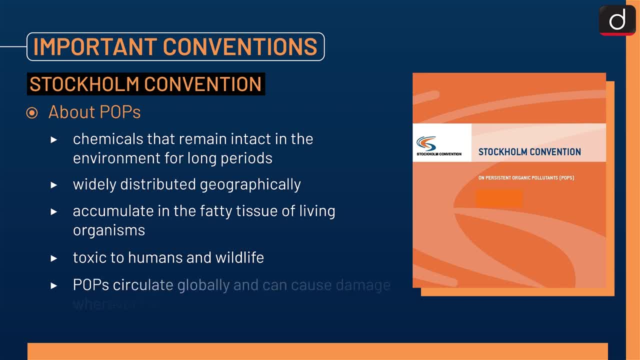 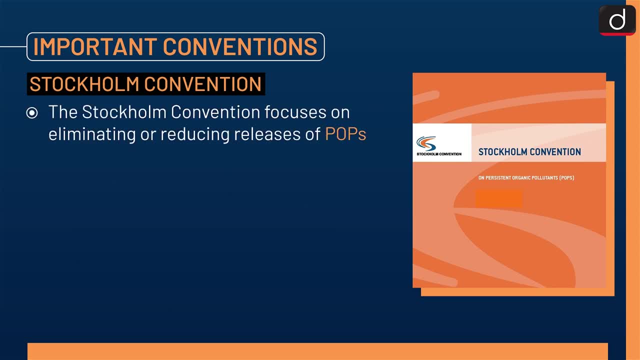 are toxic to humans and wildlife. POPs circulate globally and can cause damage wherever they travel. The Stockholm Convention focuses on eliminating or reducing releases of POPs. It sets up a system for tackling and controlling pollution of the environment. This system enables the 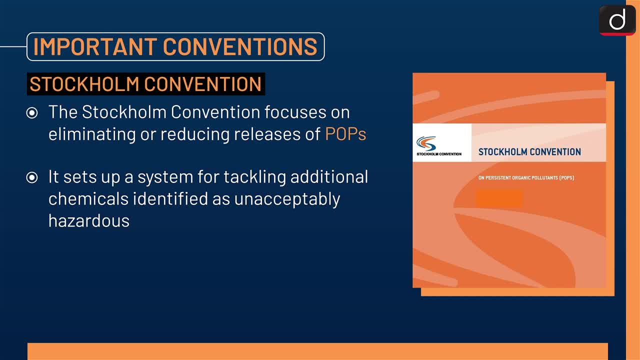 tackling additional chemicals identified as unacceptably hazardous. Ultimately, the Convention points out the way to a future free of dangerous POPs and promises to reshape our economy's reliance on toxic chemicals. Aims of the Stockholm Convention include: eliminate dangerous POPs, support the transition to. 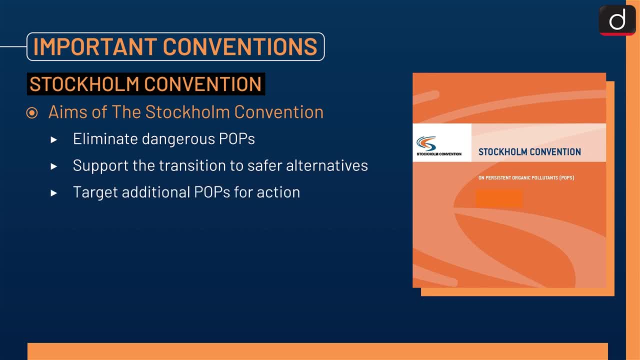 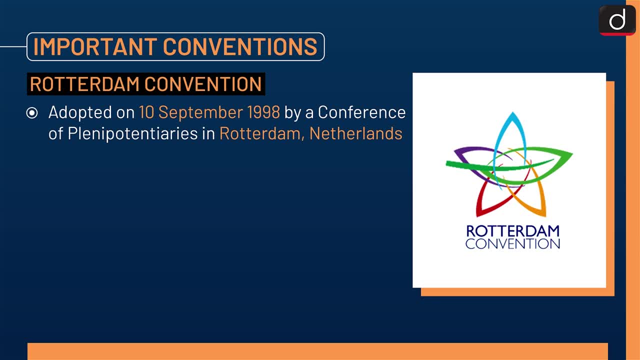 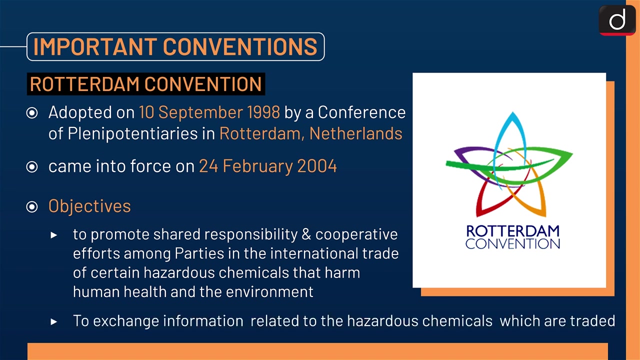 The Conference of Plenipotentiaries in Rotterdam, Netherlands. It came into force on 24 February 2004.. Objectives of Rotterdam Convention are to promote shared responsibility and cooperative efforts among parties in the international trade of certain hazardous chemicals that harm human health and the environment, and to exchange information related to the hazardous 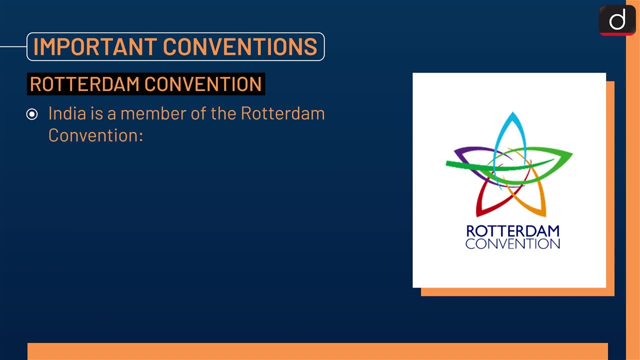 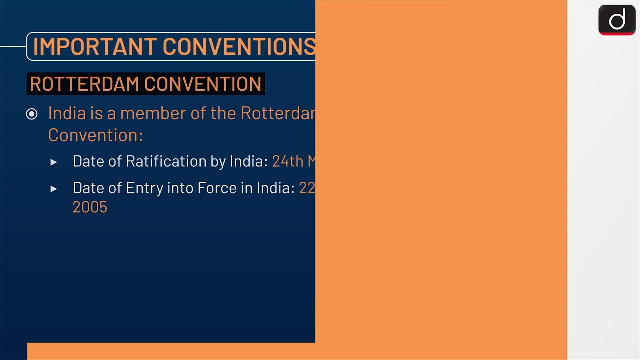 chemicals which are traded. India is a member of the Rotterdam Convention, in which the date of ratification by India is 24 May 2005 and the date of entry into force in India is 22 August 2005.. Next is CITES. 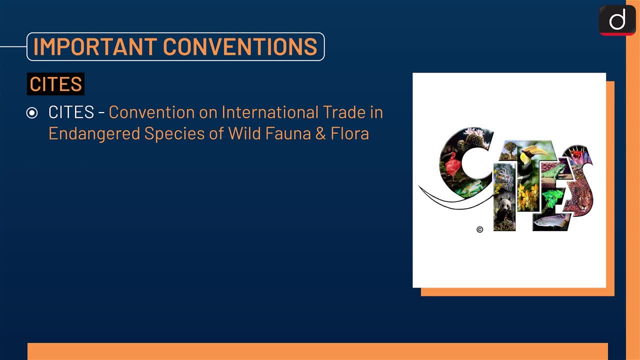 CITES is Convention on International Trade in Endangered Species of Wild Fauna and Flora. It is an international agreement between governments. The main aim of CITES is to ensure that the international trade in specimens of wild animals and plants does not threaten their survival. 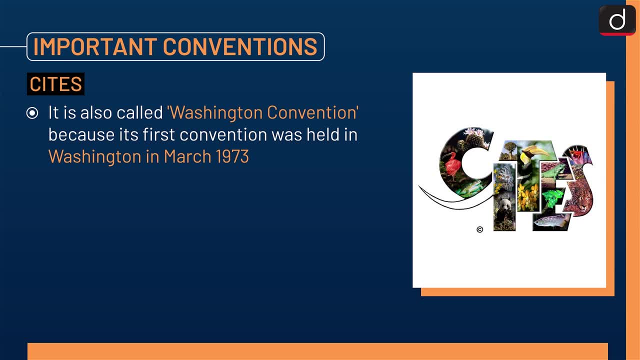 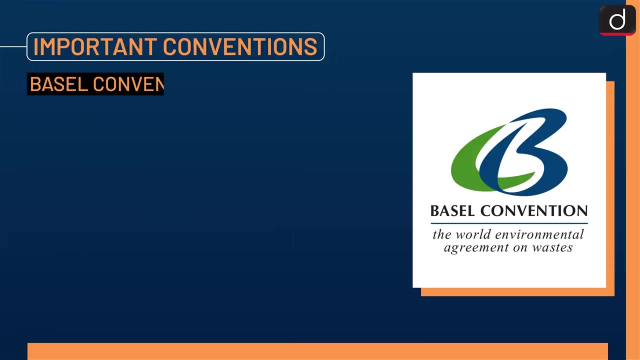 It is also called Washington Convention because its first convention was held in Washington in March 1973.. CITES is legally binding on the parties and it entered into the force on 1 July 1975.. Next is BESEL CONVENTION. BESEL Convention was adopted on 22 March 1989 by the Conference of Plenty Potentiaries. 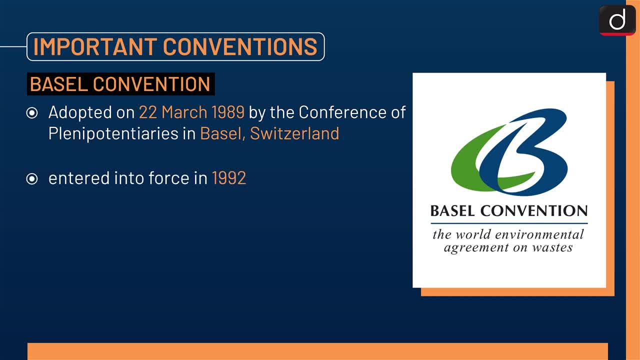 in BESEL, Switzerland. This convention entered into force in 1992.. India signed this convention on 15 March 1990 and it came into force in India in 1992.. Objectives of BESEL Convention are to control transboundary movements of hazardous wastage. 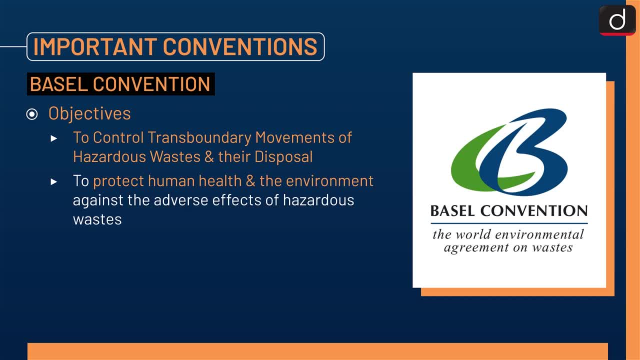 to protect human health and the environment against the adverse effects of hazardous waste, to promote clean environment protection by managing waste disposal, to reduce hazardous wastes and to create a regulatory system to check the transfer of hazardous waste. This convention includes toxic or poisonous, explosive, corrosive, inflammable, ecotoxic. 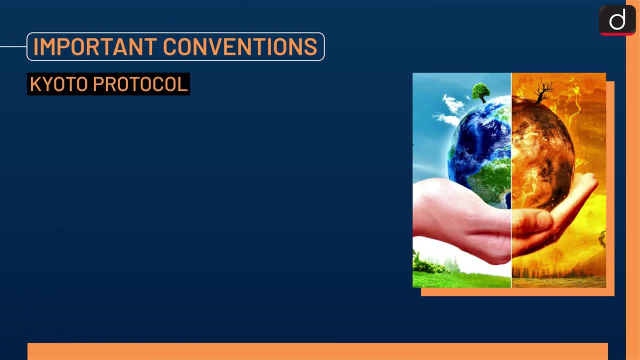 infectious waste, etc. Next is Kyoto Protocol. Kyoto Protocol was adopted on 11 December 1997 and it entered into the force on 16 February 2005.. Currently, there are 192 parties to the Kyoto Protocol. It is an international agreement under UNFCCC. 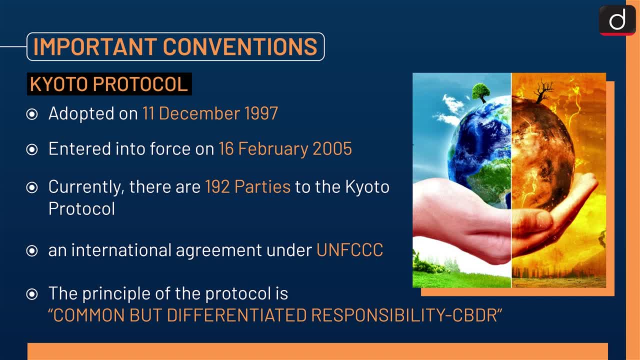 The principle of the protocol is common but differentiated responsibilities. The principle of the protocol is common but differentiated responsibilities. The principle of the protocol is common but differentiated responsibilities. I quote on the theirarticle cbdr. I quote on the theirarticle cbdr: 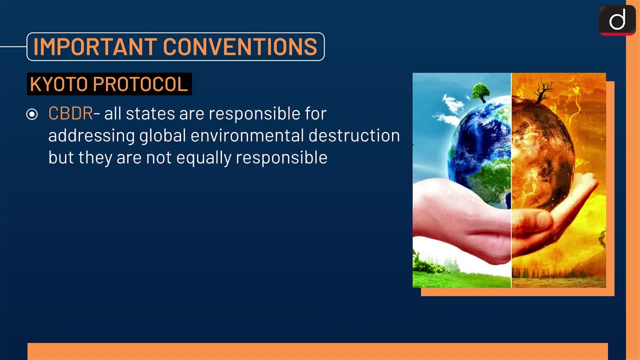 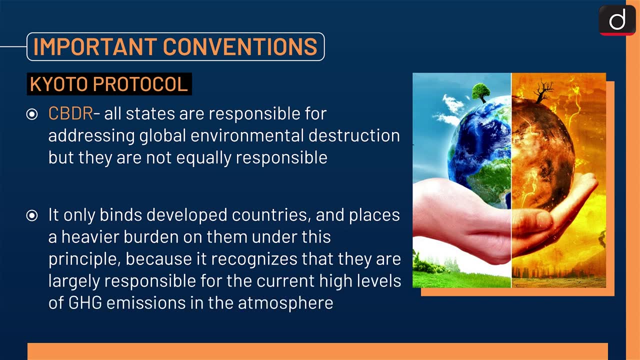 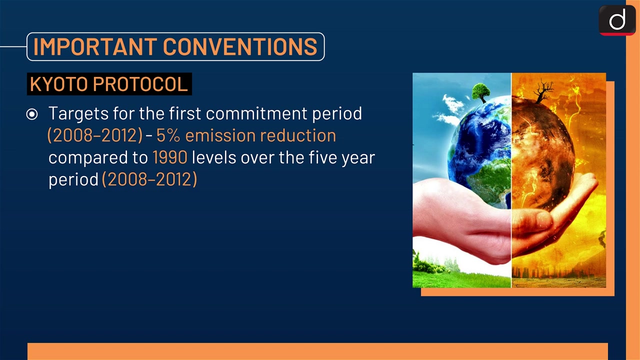 infringed, pursued the that the at debut is not limited to the public or ela, excited whoever weapons protections And countries and places a heavier burden on them under this principle. that is, 2008 to 2012, 5% emission reduction compared to 1990 levels over. 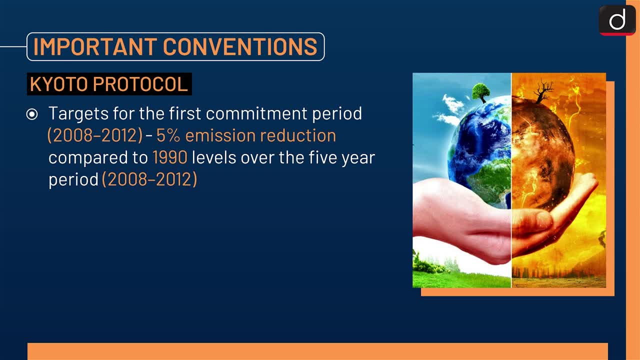 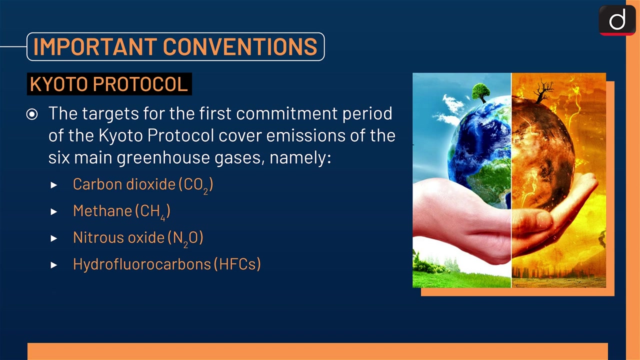 the five-year period, that is, 2008 to 2012. the targets for the first commitment period of the Kyoto Protocol cover emissions of the six main greenhouse gases, namely carbon dioxide or co2, methane or ch4, nitrous oxide or n2o, hydrofluorocarbons or HFCs, perfluorocarbons or PFCs, and sulfur. 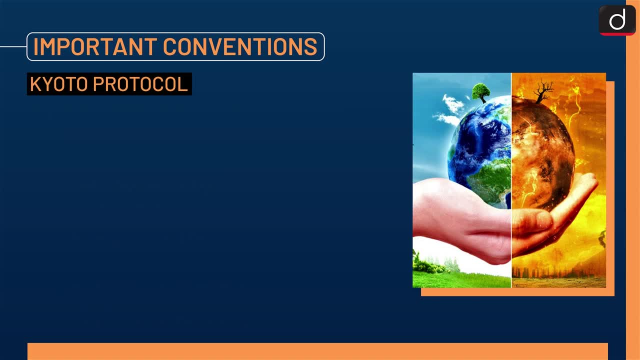 hexafluoride or sf6. now let's discuss the Doha amendment. in Doha, Qatar, on 8 December 2012, the Doha amendment to the Kyoto Protocol was adopted for a second commitment period, that is, 2013 to 2020. the Doha amendment has not yet entered. 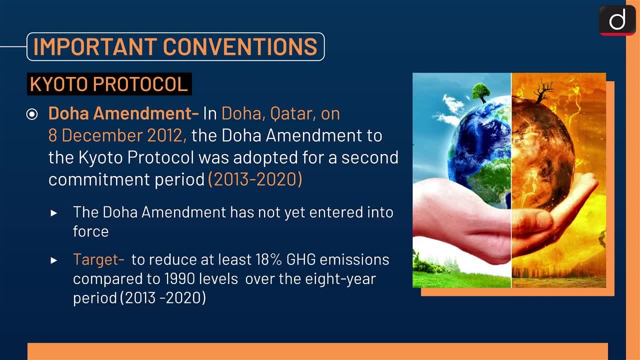 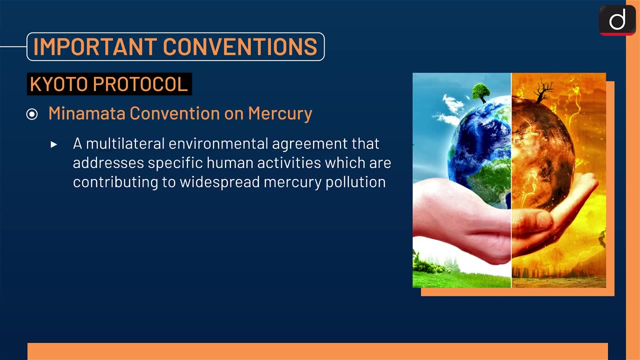 into force. its target is to reduce at least 18% GHG emissions, compared to 1990 levels, over the eight-year period, that is, 2013 to 2020. next convention is Minamata Convention on mercury. it is a multilateral environmental agreement that addresses specific human activities which are contributing to. 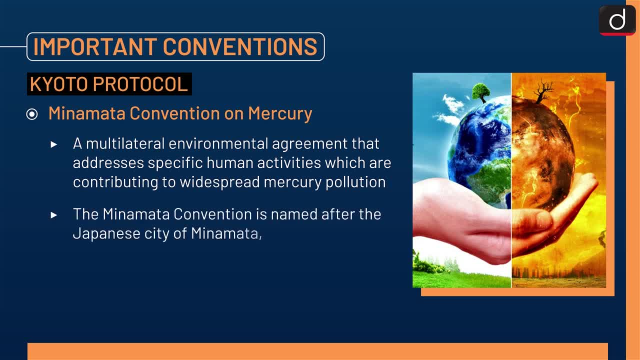 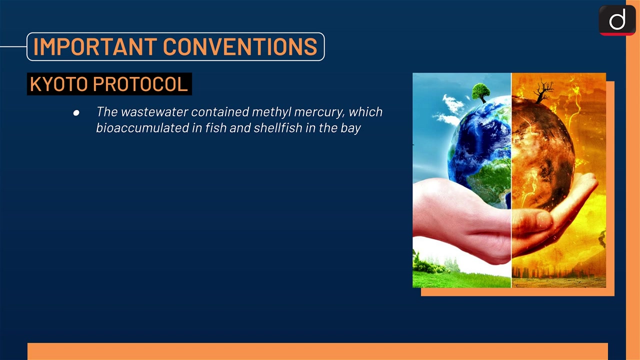 widespread mercury pollution. the Minamata Convention is named after the Japanese city of Minamata. this city experienced a severe, decades long incidence of mercury poisoning. the wastewater from the chemical factory was discharged into the Minamata Bay. the wastewater contained methyl mercury, which bio-accumulated in fish and shellfish into the bay. local people, who 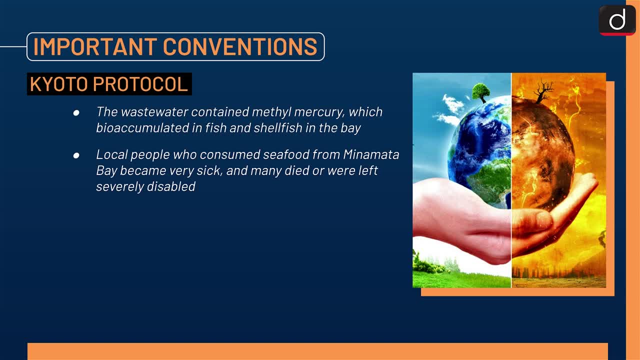 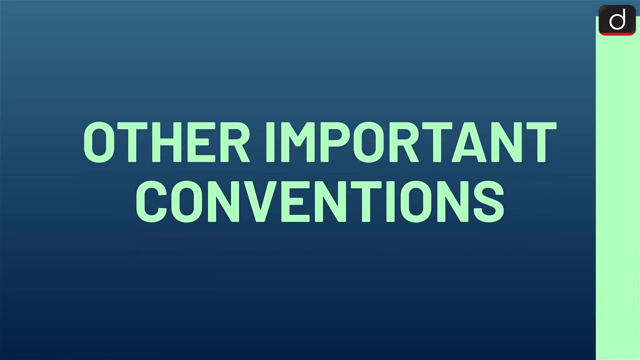 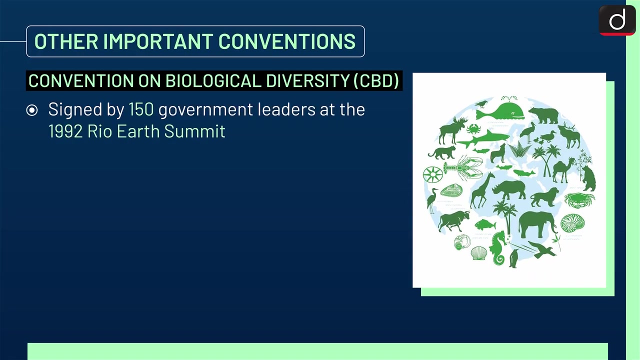 consumed seafood from Minamata Bay became very sick and many died over left left severely disabled. the convention entered into force in 2017 and India ratified it in 2018. now let's discuss some other important conventions. first is CBD, that is, convention on biological diversity. CBD was signed by 150 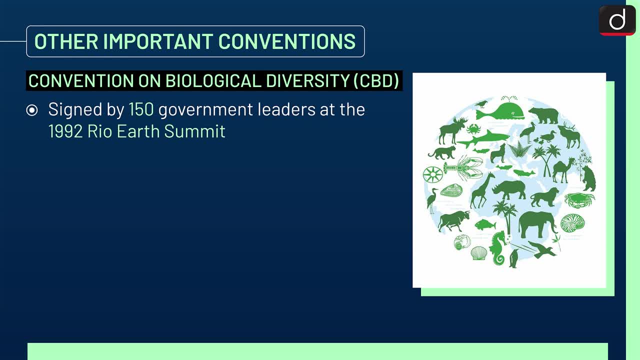 government leaders at the 1992 Rio Earth Summit and it is a legally binding convention. it entered into force on 29 December 1993. it has three main objectives: the conservation of biological diversity, the sustainable use of the components of biological diversity and the fair and equitable 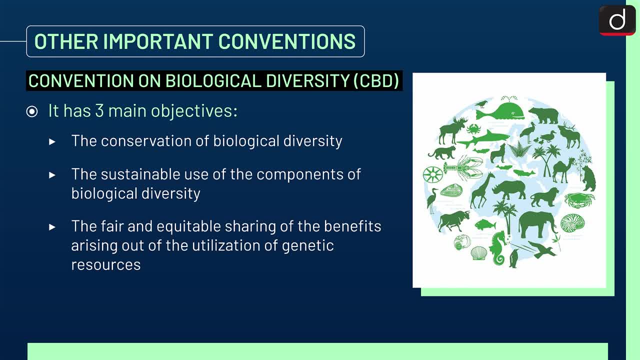 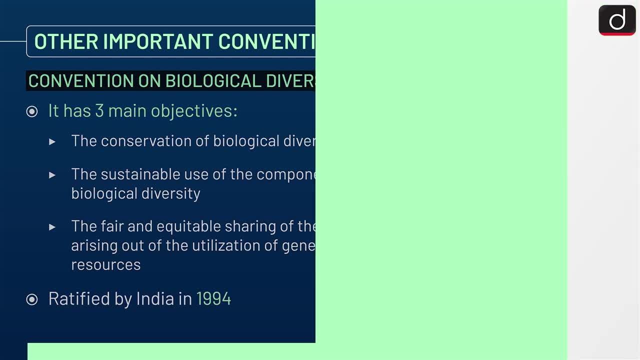 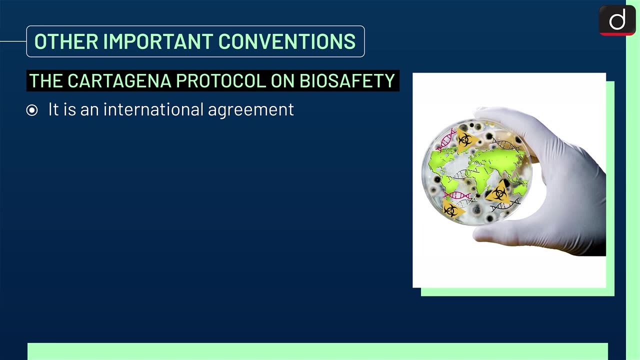 sharing of the benefits arising out of the utilization of genetic resources. it was ratified by India in 1994. next is the Cartagena Protocol on Biosafety. It is an international agreement and it aims to ensure the safe handling, transport and use of living modified organisms, or LMOs. LMO is a living 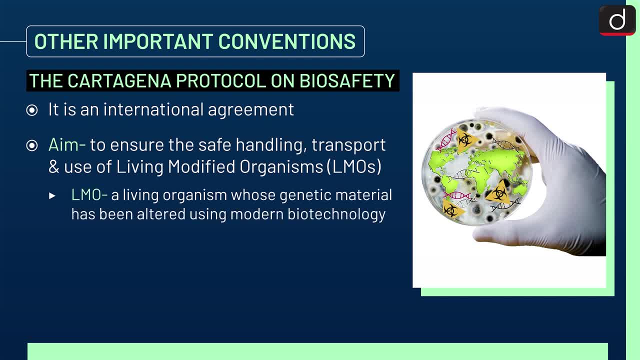 organism whose genetic material has been altered using modern biotechnology. LMO are a subset of Genetically Modified Organisms or GMOs. A GMO is any organism whose genetic material has been altered using modern biotechnology. LMO may have adverse effects on biological 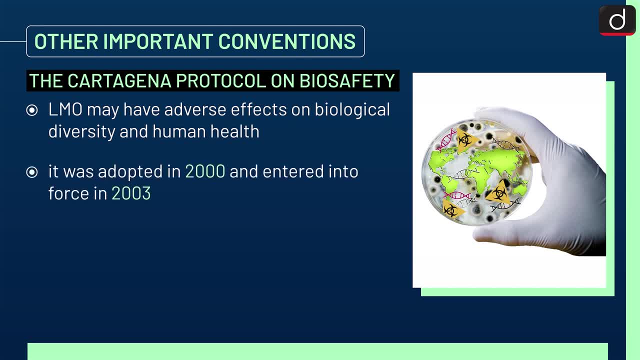 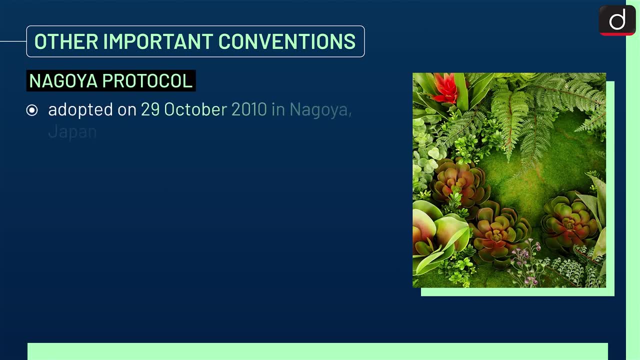 diversity and human health. It was adopted in 2000 and entered into force in 2003.. Next is Nagoya Protocol. It was adopted on 29th October 2011.. It entered into force on 12th October 2014.. It is a supplementary agreement to the Convention. 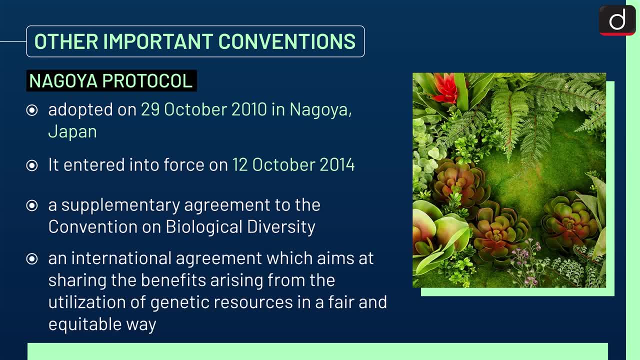 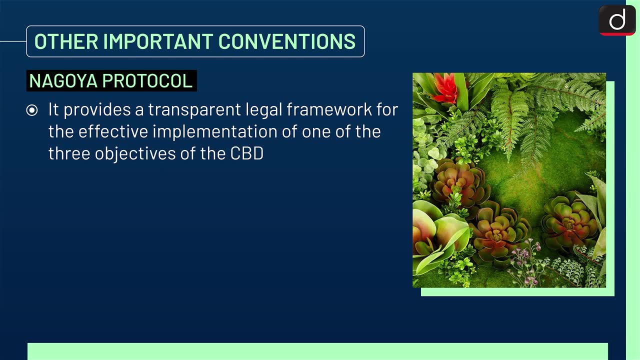 on Biological Diversity. It is an international agreement which aims at sharing the benefits arising from the utilisation of genetic resources in a fair and equitable way. It provides a transparent legal framework for the effective implementation of one of the following principles: It provides a transparent legal framework for the effective implementation of one of the following principles: 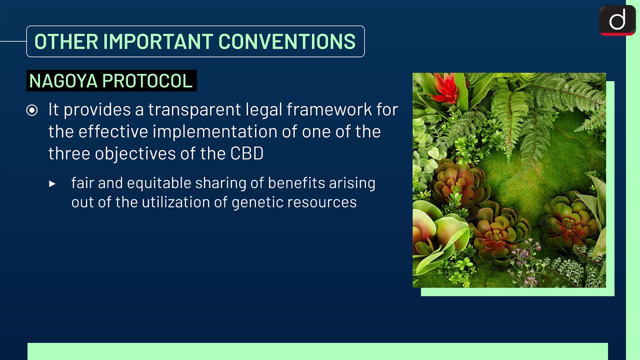 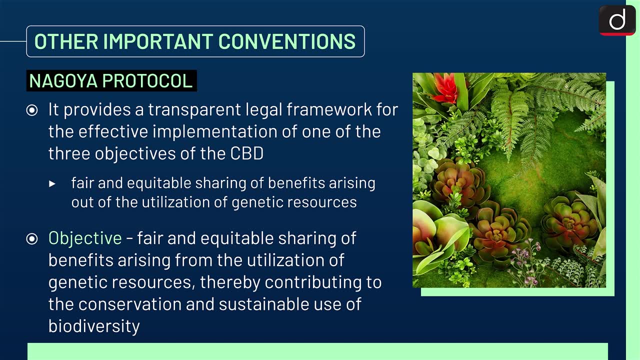 First of all, the three objectives of CBD – fair and equitable sharing of the benefits arising out of the utilisation of genetic resources. poison their animals and게요 pre 번� Odyssey of the United States. estrogen andids are not safe for live and prevent women. 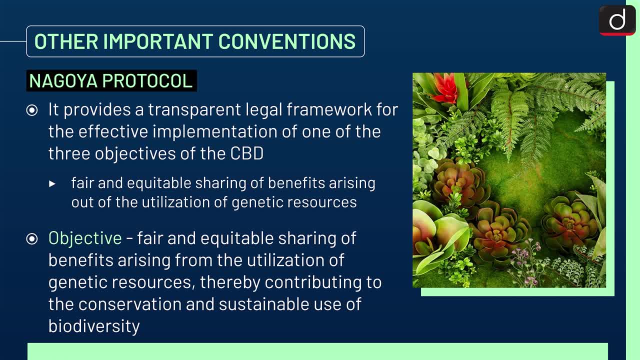 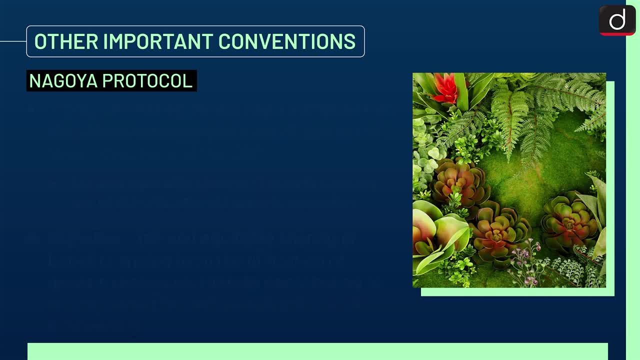 Second of all, 극성가 � Москвinky log получить Fair and equitable sharing of the benefits arising from the utilisation of genetic resources there by contradicting to the conservation and threatening to use of biodiversity. Third, the Protocol obligation sets out core obligations for its means, as contracting 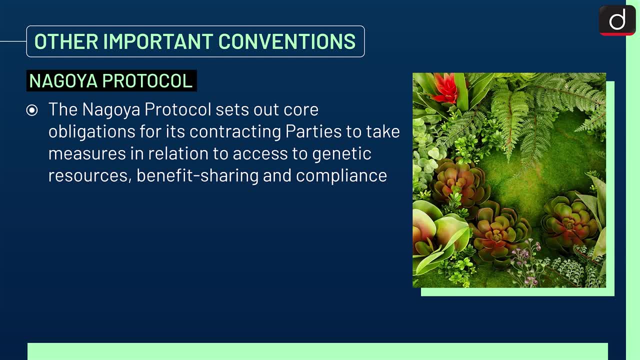 of ES parting and with Belarus, because it also has a lot of priorities for the trials. Genetic measures in relation to access to genetic resources, benefit sharing and compliance. Genetic resources refers to any biological material which contains genes and or metabolic material that may be derived from genes. 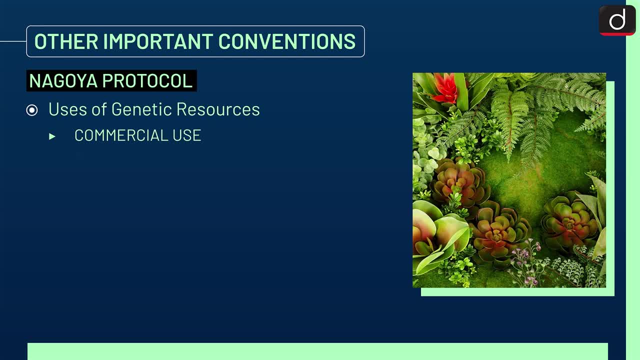 Uses of genetic resources are. first is commercial use. Companies can use genetic resources to develop speciality enzymes, enhanced genes or small molecules. These can be used in crop protection, drug development and the production of specialized chemicals In the pharmaceutical industry. for example, the US National Cancer Institute worked with 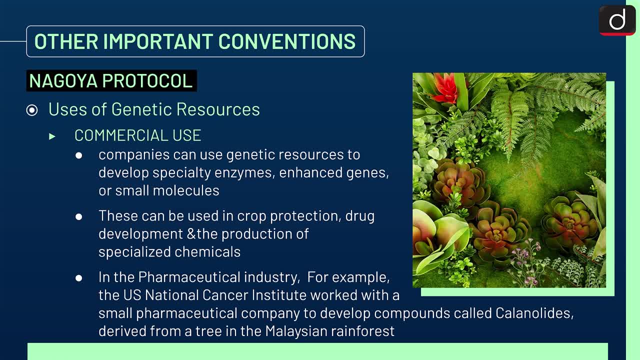 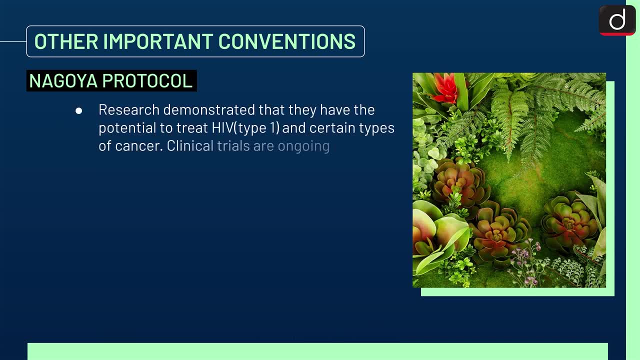 a small pharmaceutical company to develop compounds called calanolides derived from a tree in the Malaysian rainforest. Research demonstrated that they have the potential to treat HIV type 1 and certain types of cancer. Enel trials are ongoing Now. the non-commercial uses include genetic resources can be used to increase knowledge. 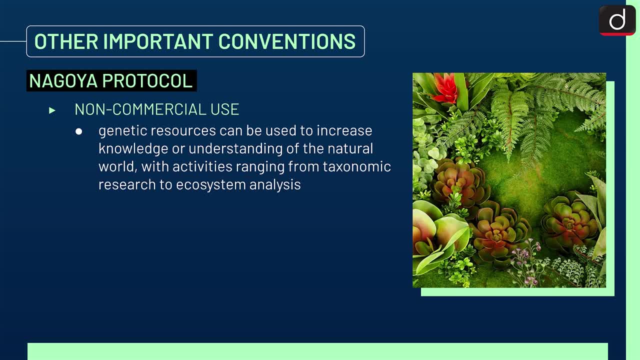 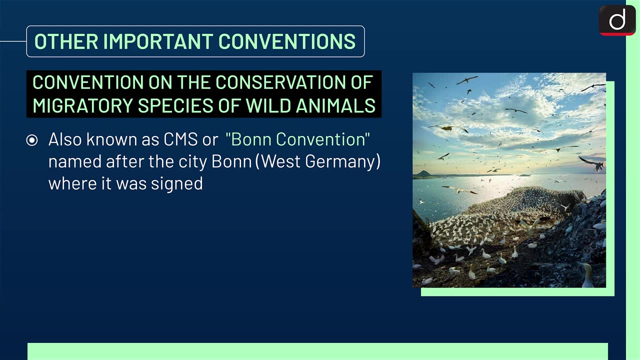 or understanding of the natural world, with activities ranging from taxonomic research to ecosystem analysis. this work is usually conducted by academic and public research institutes. Next is convention on the conservation of migratory species of wild animals. It is also known as this: A project which is Co-op, shared the genes and the disorders of natural animals, similar to all the circPCI concepts and is used for iedereen of masculinity, غر, Cheers, Westernộ, سمع and fifs and international norms of multiple species with traditional 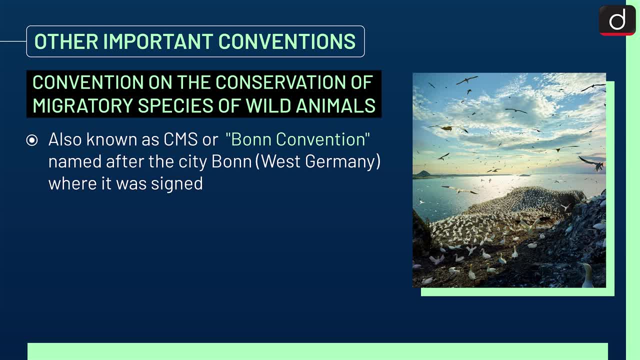 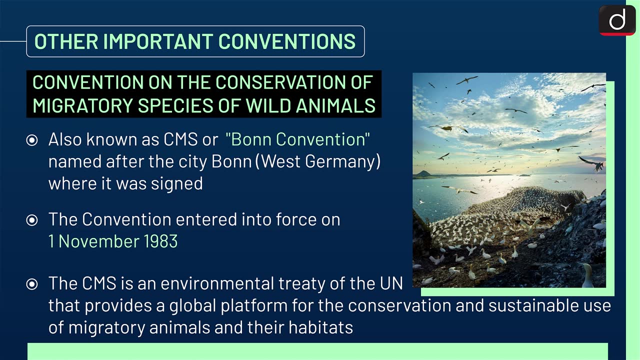 as CMS or Bonn Convention, named after the city Bonn in West Germany, where it was signed. The Convention entered into force on 1 November 1983.. The CMS is an environmental treaty of the UN that provides a global platform for the 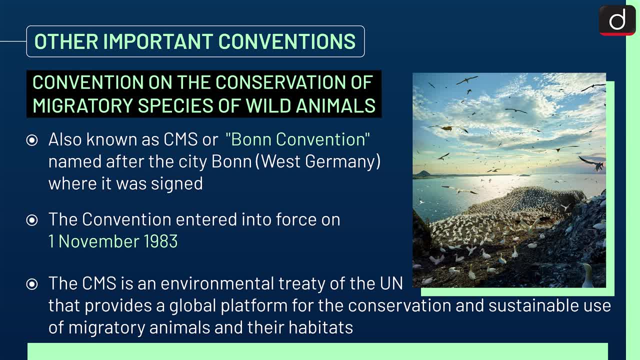 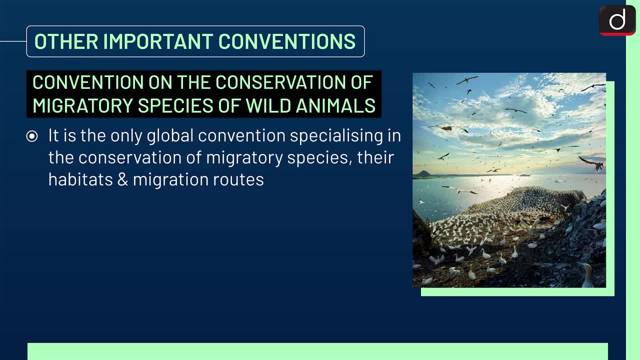 conservation and sustainable use of migratory animals and their habitats. It is the only global convention specializing in the conservation of migratory species, their habitats and migration routes. India has been a party to the CMS since 1983.. Now, lastly, let's discuss the Paris Agreement.